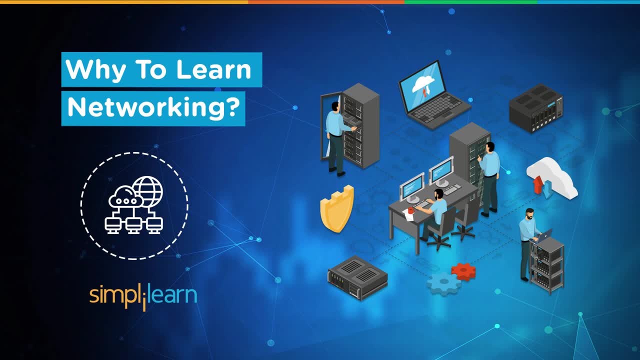 work and play. In this tutorial video, we will unveil the power and potential of networking and why it's a skill you absolutely must have. But before we begin, if these are the type of videos you would like to watch, then hit on the subscribe button and click the bell to never miss an update from Simply Learn. 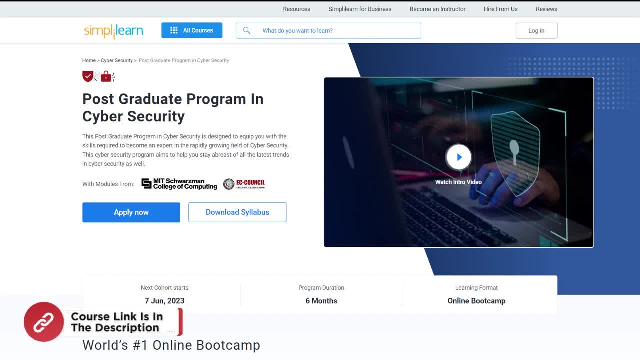 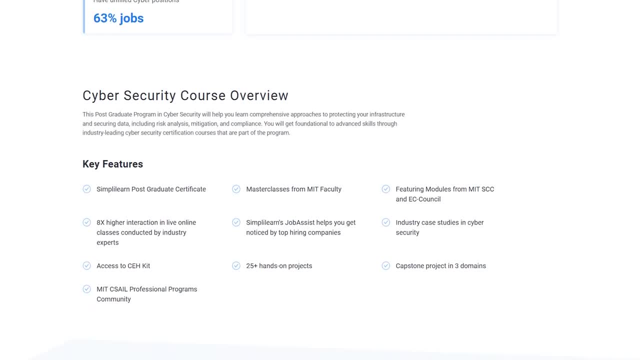 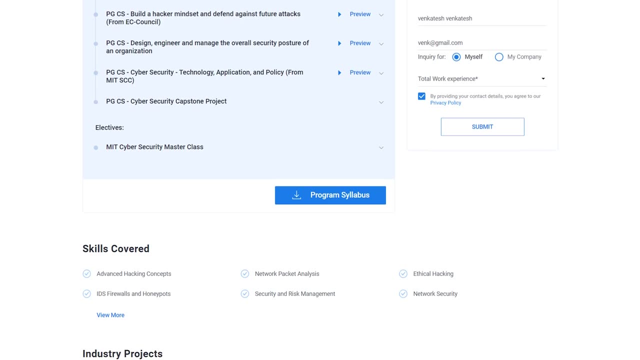 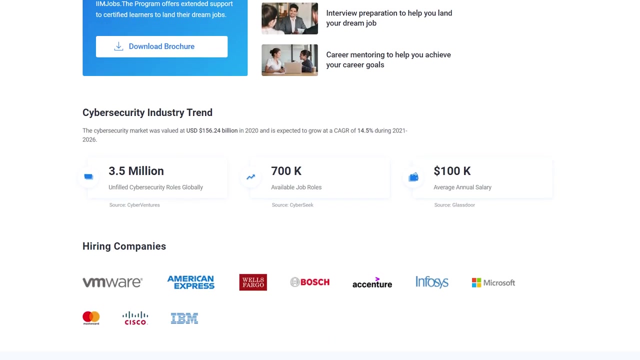 And if you are someone who is interested in building a career in cybersecurity by graduating from the best universities, or a professional who elicits to switch careers with cybersecurity by learning from the experts, then giving a shot to Simply Learn's postgraduate program in the 80's and making it to the top of the list of alls is a great option. 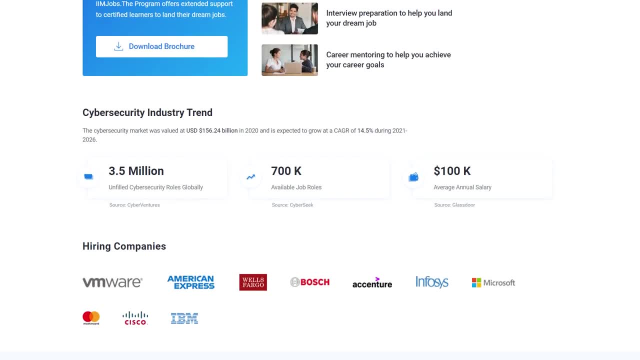 The link in the description box should navigate you to the homepage, where you can find a complete overview of the program being offered. Take action, upskill and get ahead Without further ado. let's get started with understanding why you must learn networking. 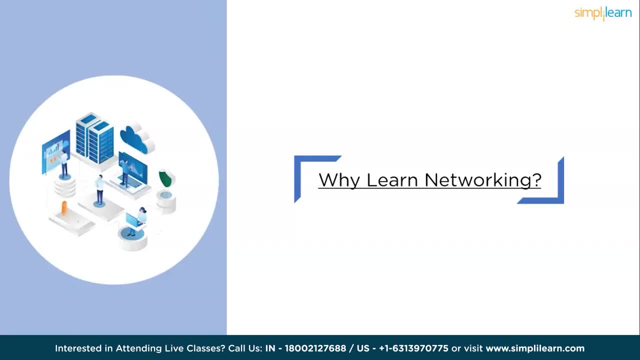 Let's get started with the first one. The first thing you need to do when learning how to do networking is to start with the very first step. In this video, we are going to show you the first step of how to do networking. To begin with, why do we need to learn networking? 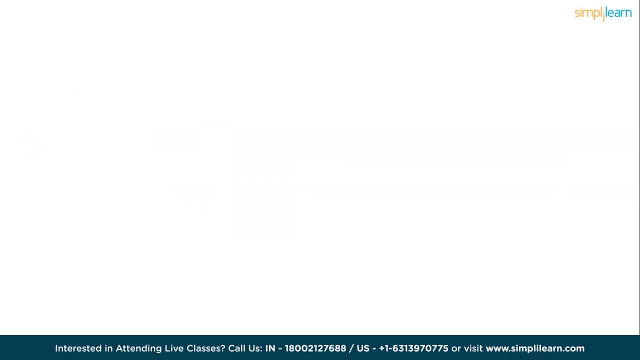 We need to dig deep and understand the importance of networking to be successful. How can you learn to learn networking in the first place? Digital fun or Internet Outsourcing or Internet Outsourcing is important to all of us on networking. Networking is closely related to other IT domains and plays a. 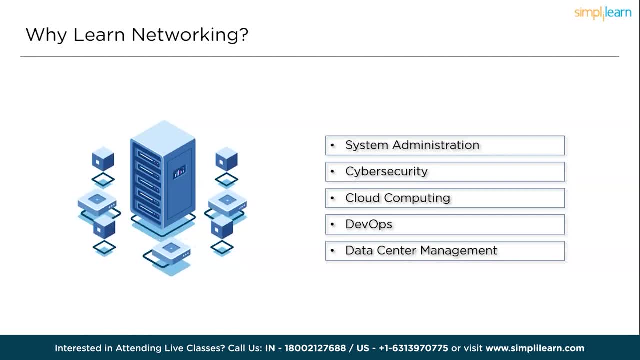 crucial role in their successful operation. Here are a few ways networking intersects with other IT roles, such as system administration, cybersecurity, cloud computing, DevOps and data center management. We will understand each one of these in detail. First, system administration: Network administrators. 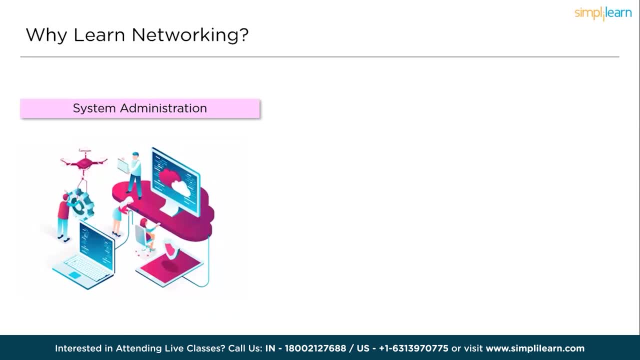 work closely with system administrators to ensure that the network infrastructure supports the smooth functioning of the systems and applications. They collaborate on tasks such as network configuration, security measures and troubleshooting network related issues. Next, we have cybersecurity. Networking and cybersecurity go hand-in-hand. Network: 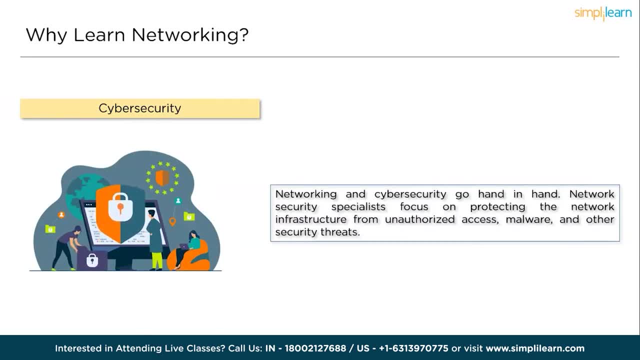 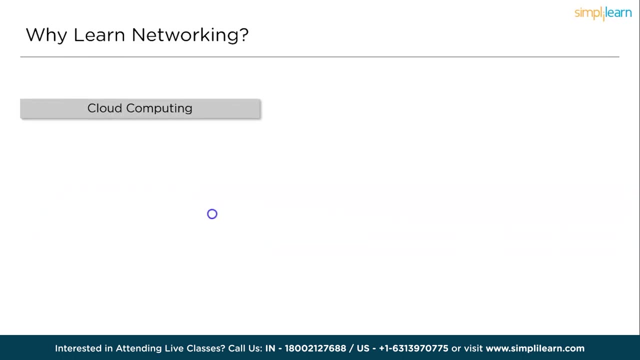 security specialists focus on protecting the network infrastructure from unauthorized access, malware and other security threats. They work alongside cybersecurity professionals to implement security measures, monitor network traffic and respond to incidents. Followed by that, we have cloud computing. Networking is an essential component of cloud computing. Cloud architects and engineers design 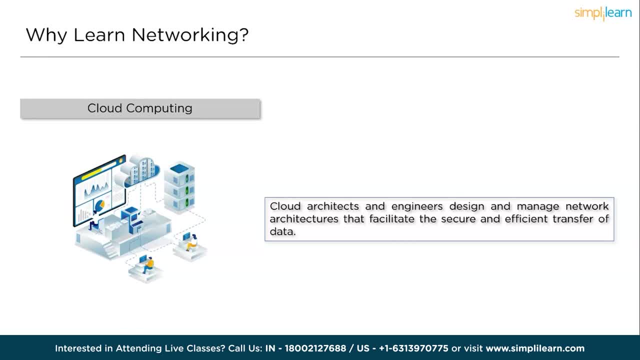 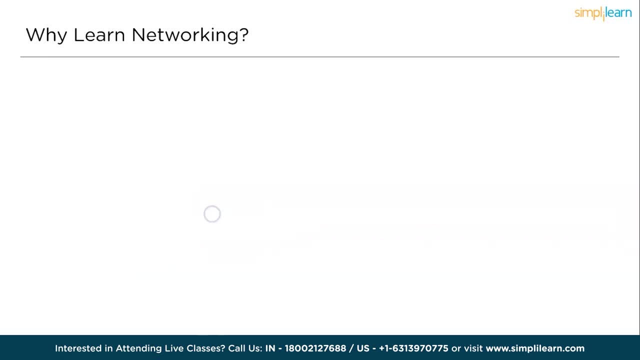 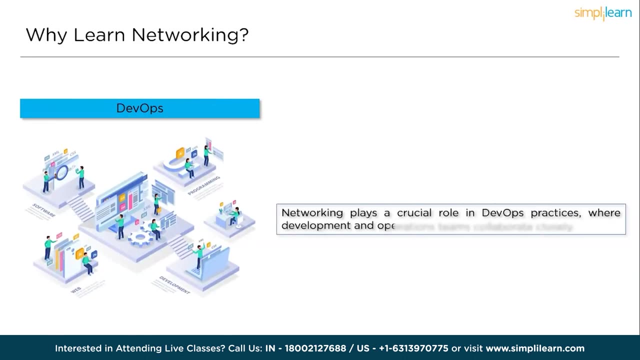 and manage network architectures that facilitate the security and efficient transfer of data between cloud services, on-premises infrastructure and end users. Next ahead we have DevOps. Networking plays a crucial role in DevOps practices where development and operations team collaborate closely. Network engineers work with DevOps professionals to design and 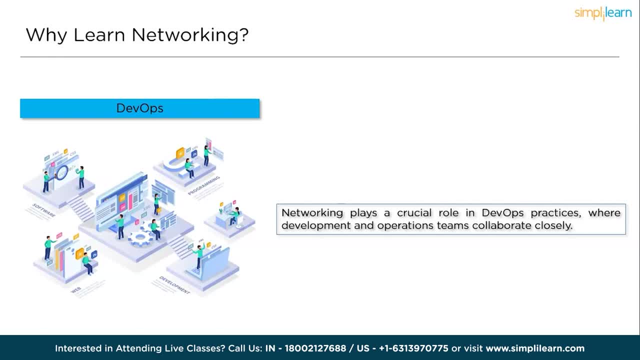 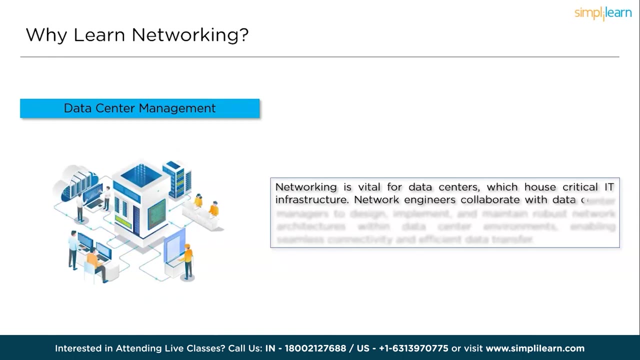 deploy networks that support continuous integration and delivery, or CICD pipelines, ensuring efficient deployment and operation of software applications. Followed by that, we have data center management. Networking is vital for data centers, which house critical ideas and solutions. Networking is an essential component of cloud computing- Cloud architectures. 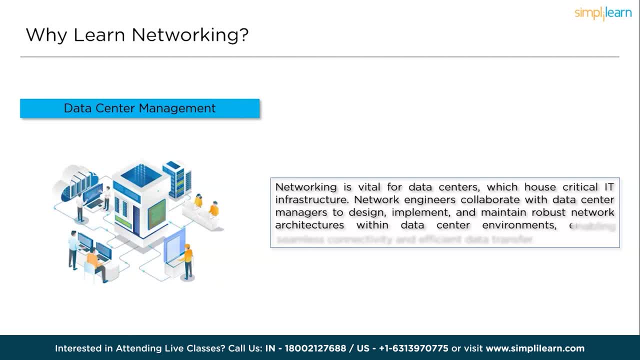 and IT infrastructure. Network engineers collaborate with data center managers to design, implement and maintain robust network architectures with data center environments enabling seamless connectivity and efficient data transfer. Networking is an integral part of IT ecosystem, collaborating with various roles to enable efficient communication. 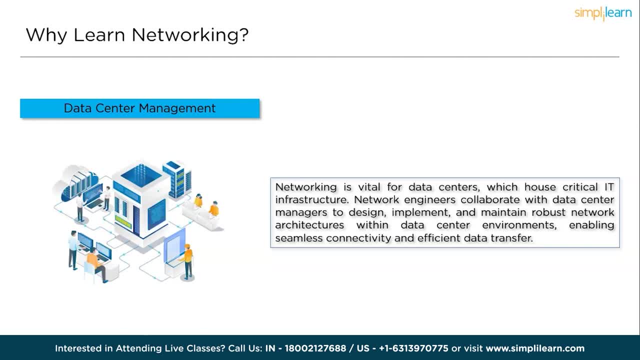 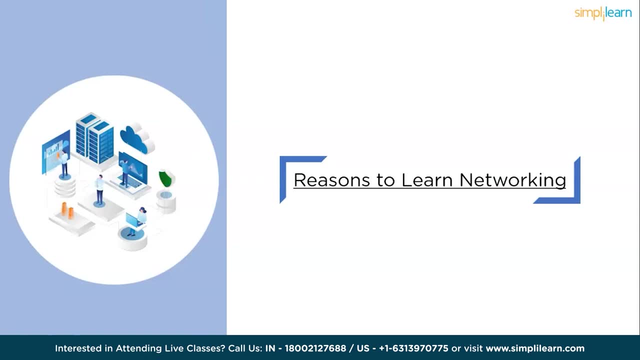 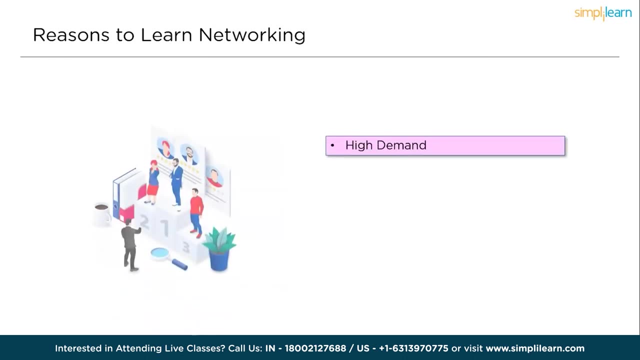 secure data transfer and reliable system operation. Apart from these, there are many compelling reasons why you should give a shot to learning the fundamentals of an IT ecosystem. Following reasons are: first, high on demand. Networking skills are on high demand, offering excellent job prospects and long-term career scalability. Followed by that, we have 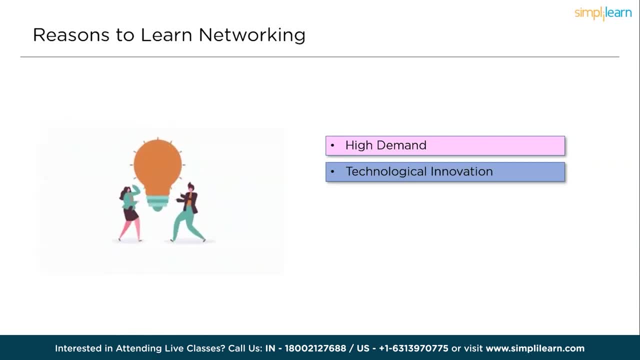 technological innovation. Networking is the forefront of technological advancements, providing opportunities to work with cutting edge technologies and shape the future. Next ahead, we have the global connectivity. Networking enables you to connect with people, businesses and ideas on a global scale, fostering collaborations and making a tangible impact on 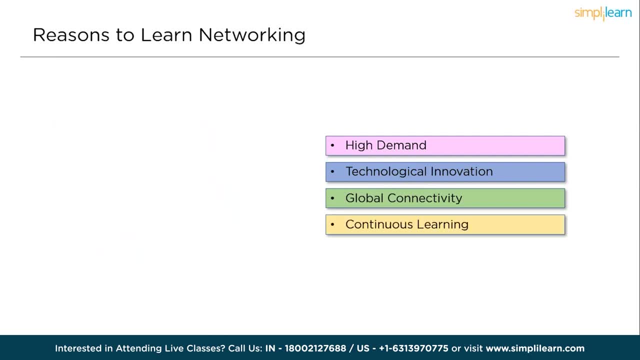 the society. Next on the docket is continuous learning. The field of networking is dynamic and ever-evolving, offering constant learning opportunities to stay ahead of the curve and expand your skill set. And lastly, we have competitive advantage: Possessing strong network. 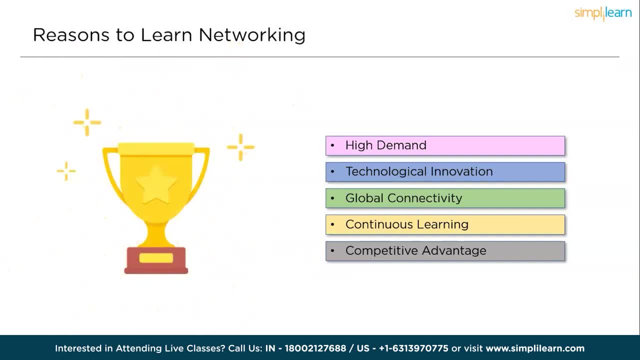 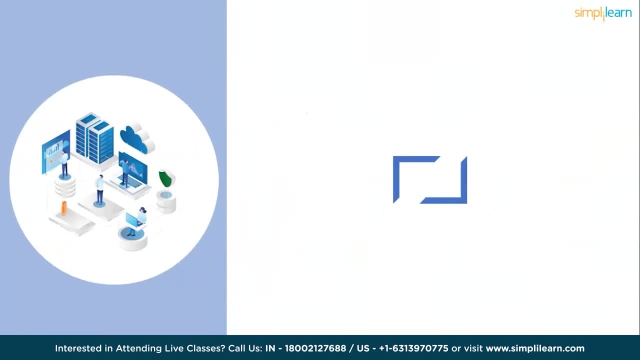 skills gives you a competitive edge, as businesses rely on reliable and secure networks to thrive in the digital age. Having known about the importance and reasons to learn networking, let's proceed with the most important aspect of networking as a career, that is, salary of a 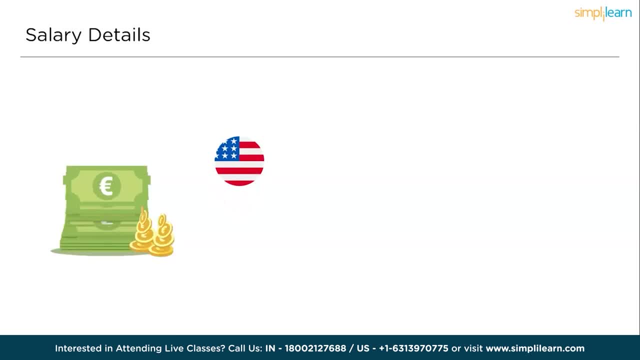 network engineer. Entry-level networking engineers in the United States of America can earn an annual salary ranging from $50,000 to $90,000 per annum, whereas on the senior level, the senior networking engineers or those in leadership positions can earn salaries exceeding. 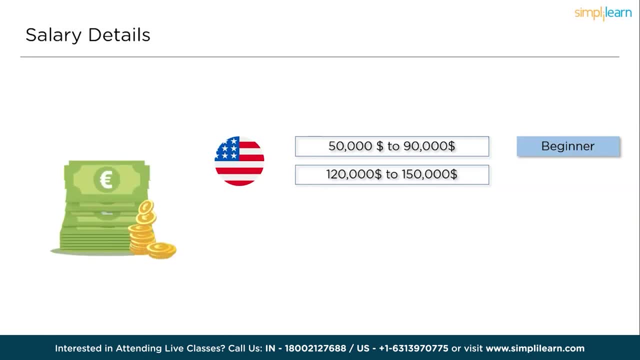 $120,000 to $150,000 or more. An entry-level networking engineer in India can expect to earn an annual salary around $6 to $12 lakhs per annum. A senior or highly experienced network engineer can earn salaries ranging from $12 lakhs to $20 lakhs per annum. 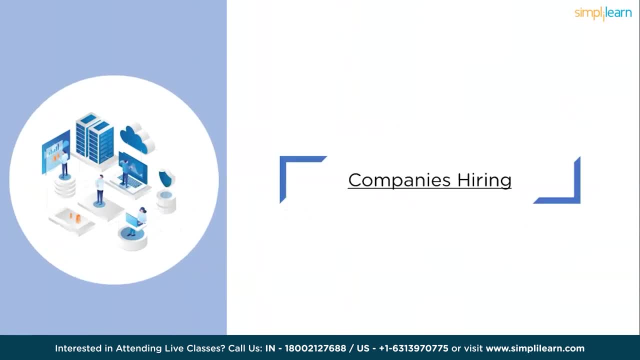 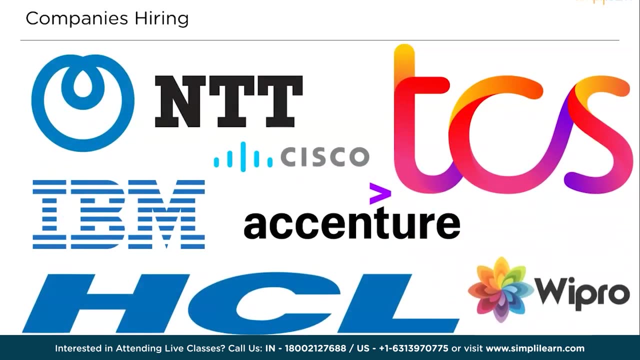 Some of the top companies hiring network engineers include the following: NTT, Cisco, TCS, HCL, IBM, HP, Accenture and Wipro. Before we end this video, let's take a minute to hear from our learners who have experienced massive success in their careers. 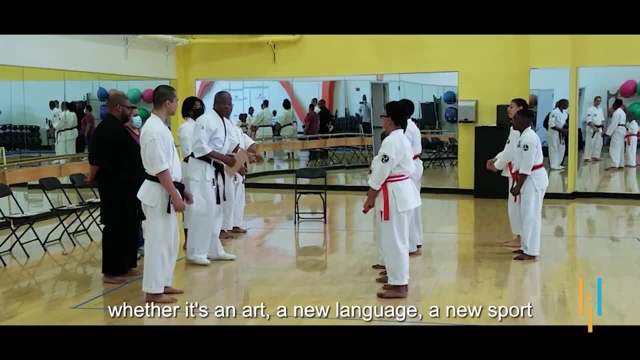 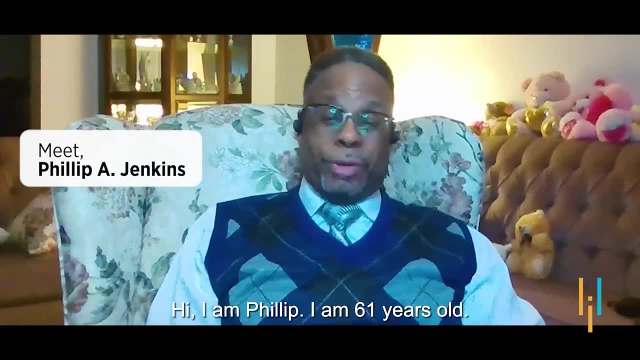 You're never too old to learn anything new, whether it's an art, a new language, a new sport or learning new skills to advance your career. Hi, I'm Philip. I'm 61 years old and last year I upskilled with SimpliSkillscom. If you're interested in learning new skills, you can. 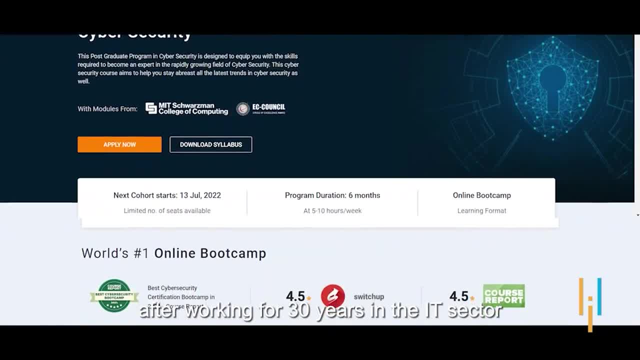 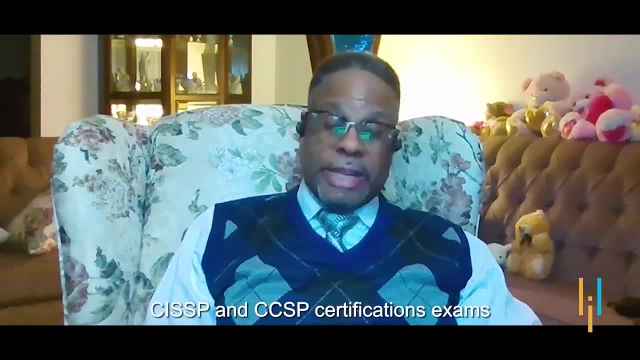 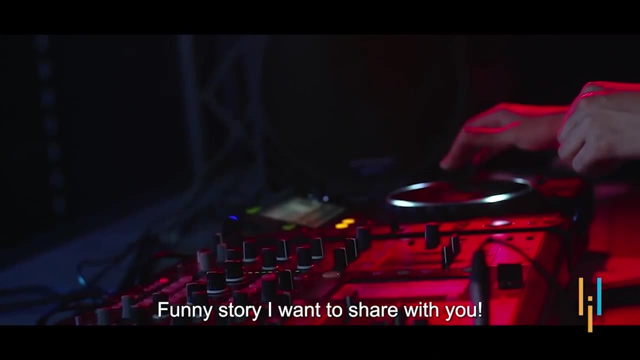 sign up for the SimpliLearns postgraduate program in cybersecurity. after working 30 years in the IT sector in various different profiles, I'm happy to tell you that I was able to clear and pass my CISSP and CCSP certification exams on the first attempt after taking the course. A funny story. 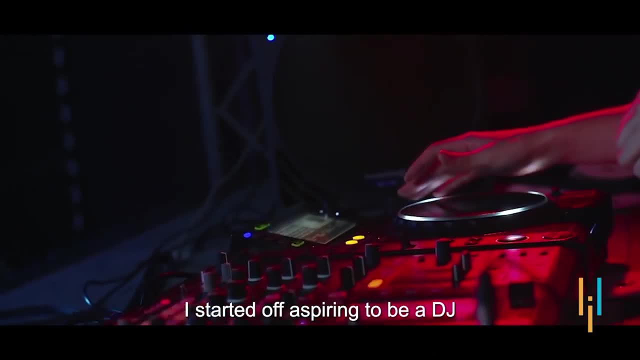 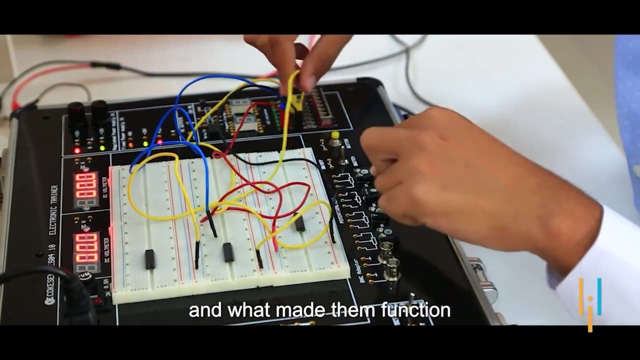 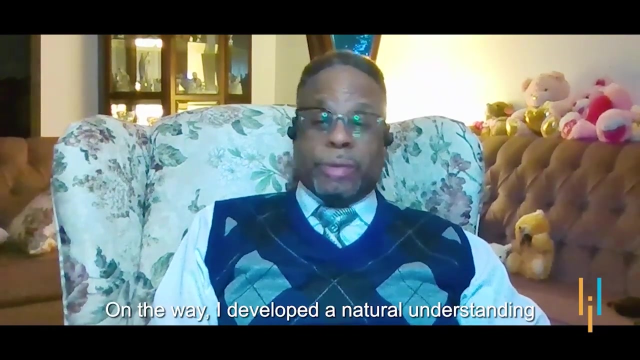 I want to share with you. I started off aspiring to be a DJ. I became interested in electronic stereo systems and how they connected and how they operate and what made them function. Four years later, I began a journey to understand and learn more about the cloud, On the way I developed a